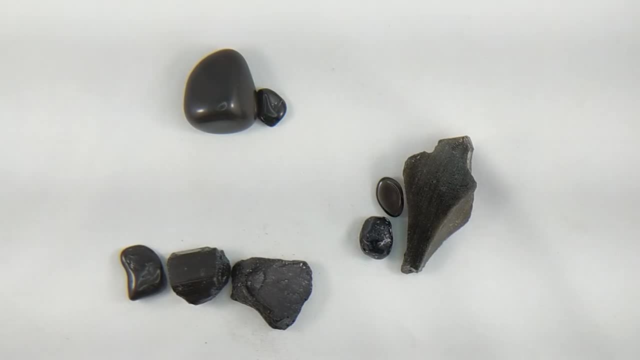 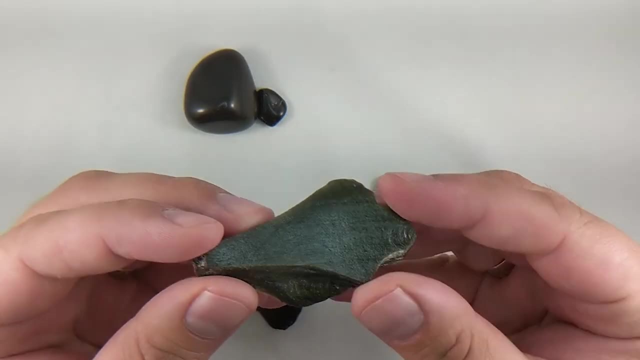 looking at them, especially when they're polished. But today we're going to show you some tips and tricks, So it makes it a little bit easier for you guys to figure out which one's which. So we're going to start with the obsidian. So obsidian is a form of volcanic glass. 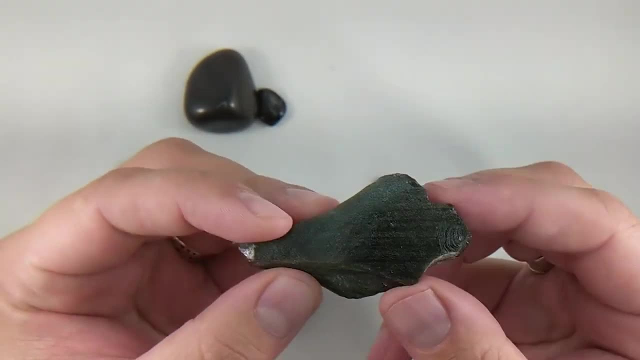 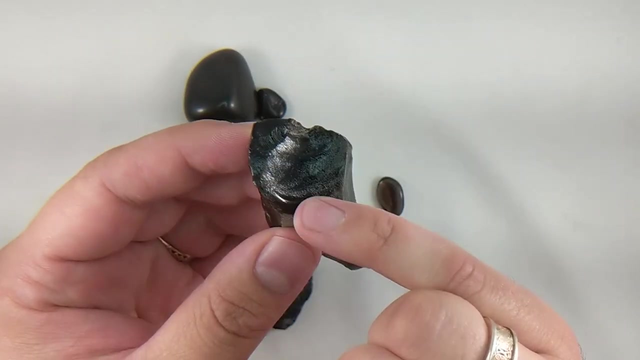 and it has some very interesting characteristics because of its being, because of it being glass, And one of the big ones, if you're looking at a piece of rock obsidian- is the spalling or the shape that it makes when it cracks. It has this really. 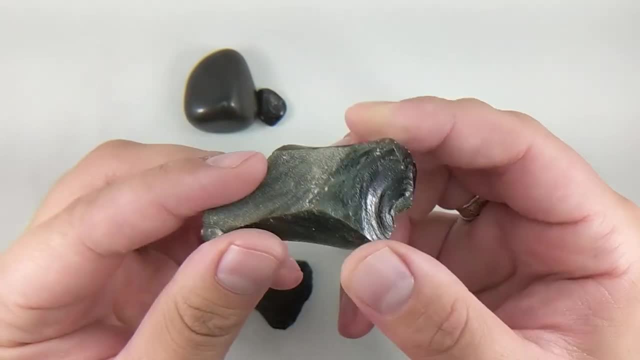 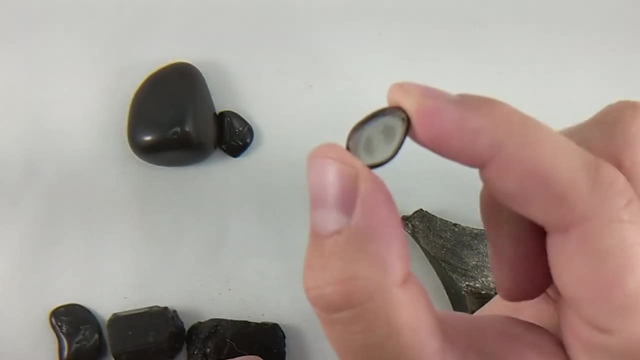 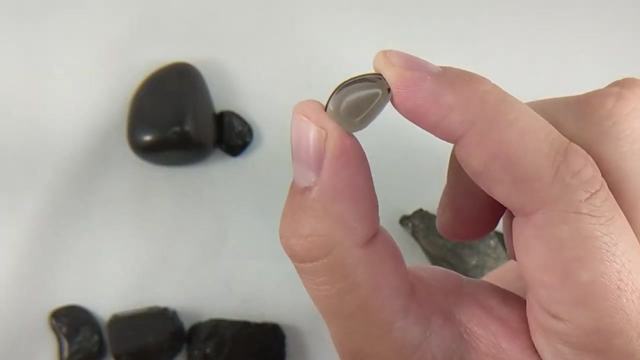 concentric ring shape when you break it. So if you accidentally drop a piece and it does this, it's obsidian. One of the other characteristics of obsidian is it can be transparent. So this piece here, which you can see probably right through, is a piece of obsidian, Whereas if 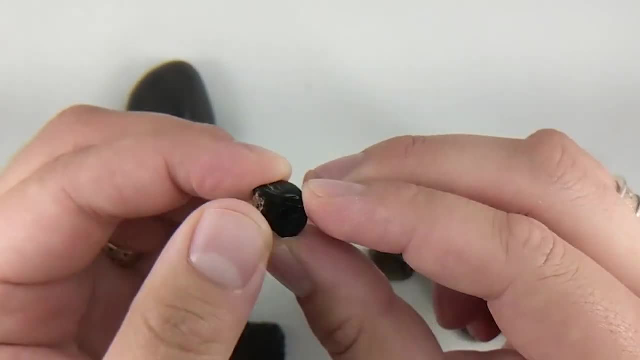 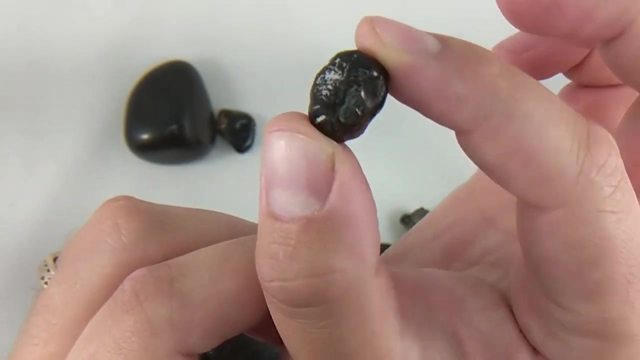 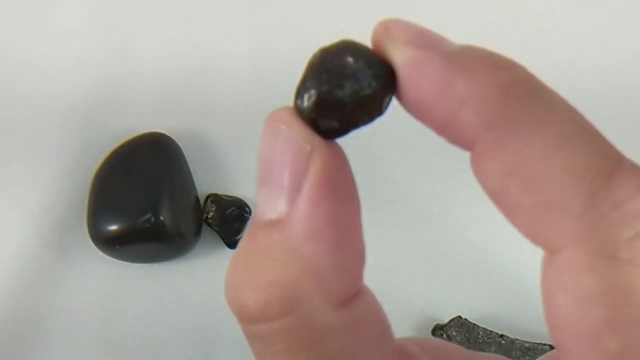 you're looking at a piece of onyx. it doesn't have any transparency to it. This here is called an Apache tear. It is a unique form of obsidian, usually from Arizona or New Mexico And, as you can see once again with the light here that it is transparent, Obsidian is. 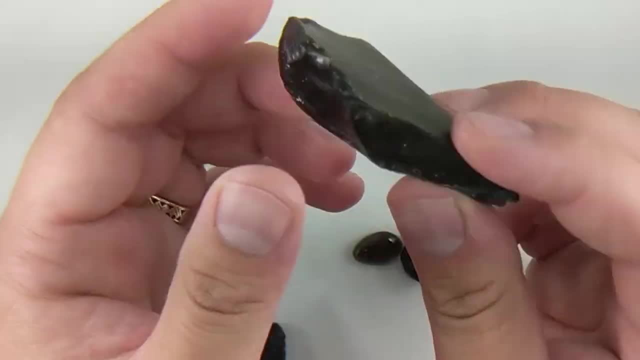 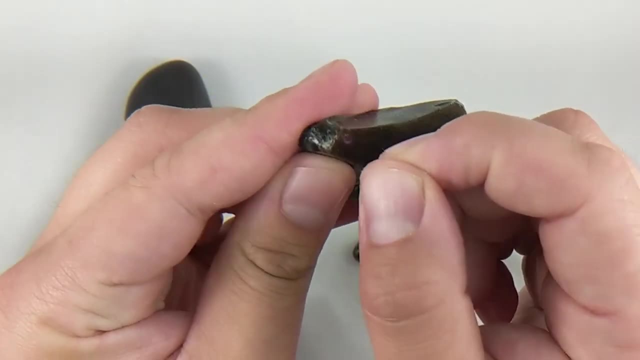 also the softest of the three. So if you have a piece of quartz, you can actually- and you don't mind scratching your piece of obsidian- you can actually scratch it. So if you take the piece of quartz, the point of it. 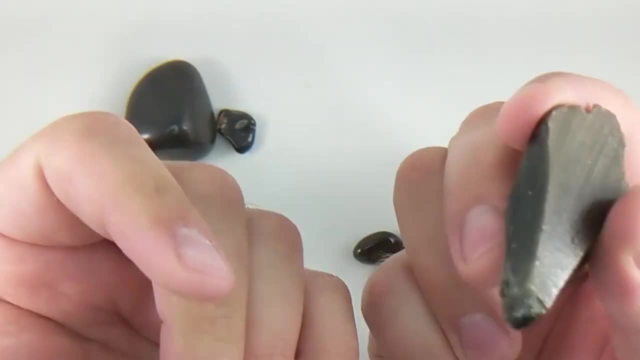 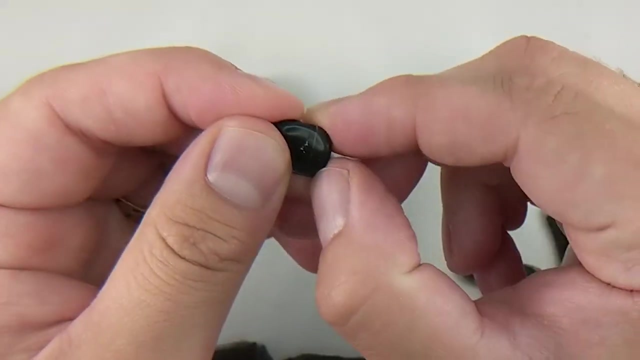 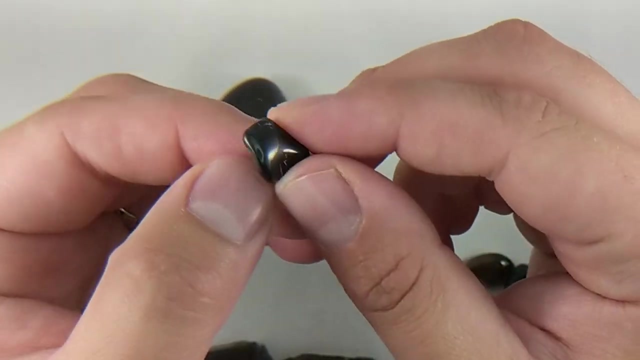 run it along it, it will actually leave a small mark in it. If it does that, it's obsidian. Moving on to onyx: here we can see that it has these lines in it. One of the characteristics of black onyx is that it will have parallel lines. So you can see, this one only has the one, but you. 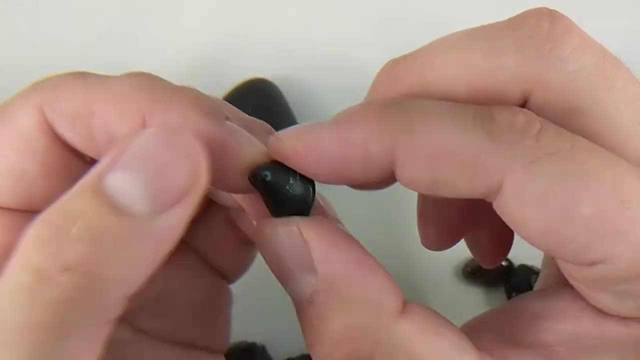 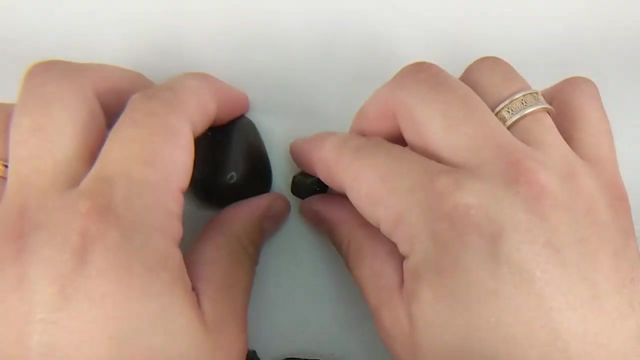 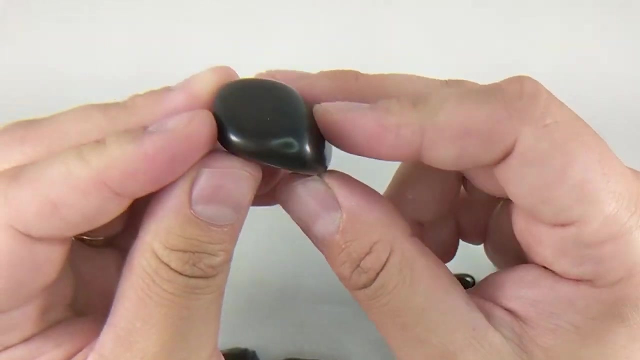 can see these tiny little lines in it And that helps you identify onyx versus obsidian. As you can see between the two of them under some good light, they're quite different. Now, sometimes onyx does come just as a black rock. This is still fairly easy to tell the difference. 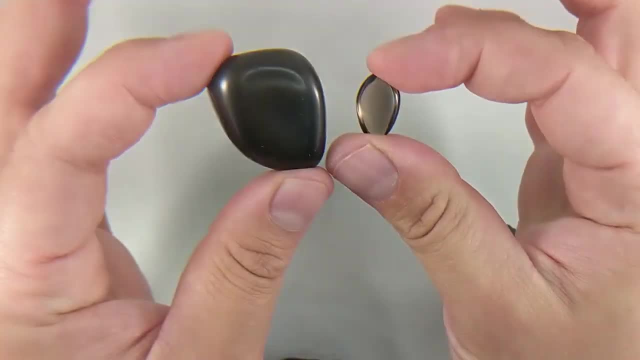 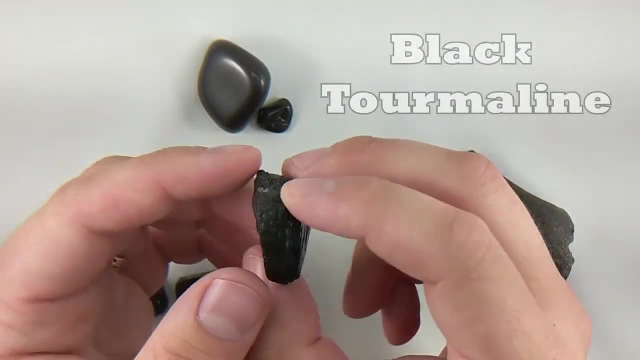 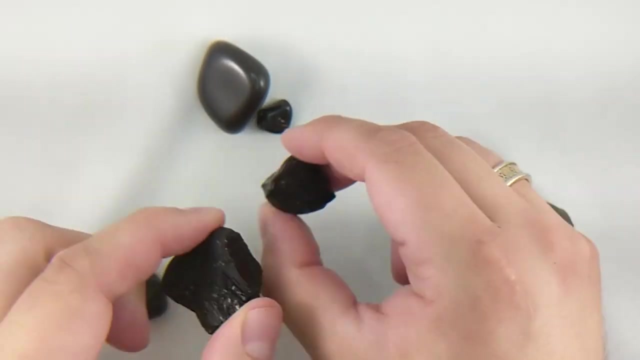 because you can still see through obsidian. usually Use your cell phone light behind the rock and you can get a good color behind it. So this is a chunk of rough black tourmaline. Now black tourmaline forms in these long, striated crystals. You can't see that great on this piece, but on